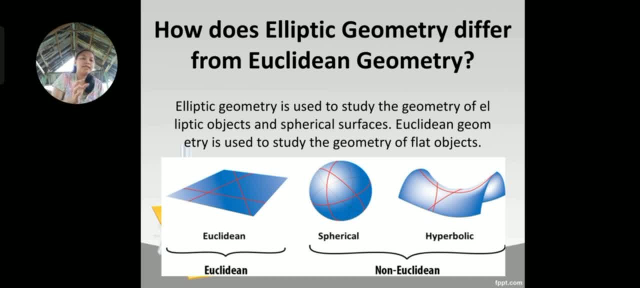 considered a flat object in Euclidean. so this and the second and third, which is this spherical and hyperbolic, are considered a non-Euclidean. so that would be all in my part, and John Michael Tavis will be the one to continue our report. thank you, I. 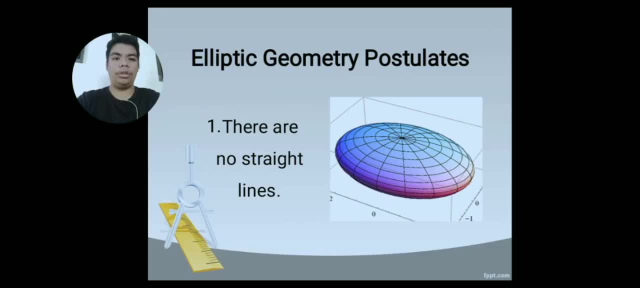 am John Michael J Tavis and I am going to continue the report of Rosanna Monsalves. elliptic geometry postulates. first postulate is there are no straight lines. any lines that is drawn in a curved surface will always be curved because the surface itself is. 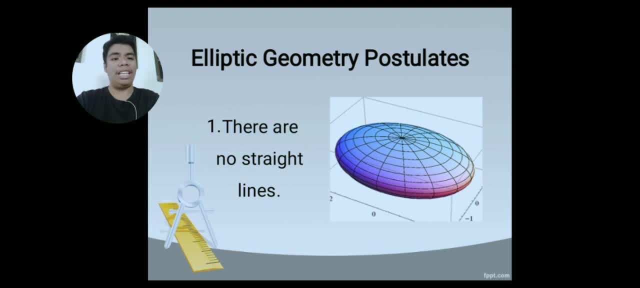 curved, since ellipse is more like a flattened circle and we all know, and it is obvious, that the circle is composed of curved lines. therefore, the ellipse is also composed of curved lines and there are no straight lines we can see in an ellipse. there are no parallel lines as well. if we are going to look closely here in the 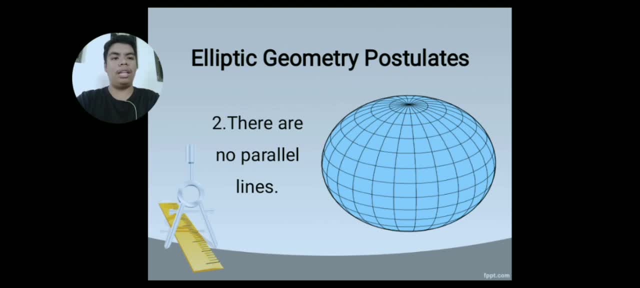 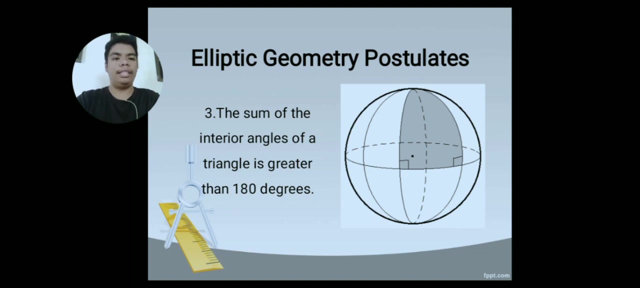 figure at the right, we can see that all the lines always intersect from each other. we cannot see a line that is parallel to each other, since all lines always cross from each other at some point. the sum of the interior angles of a triangle is greater than 180 degrees, since the 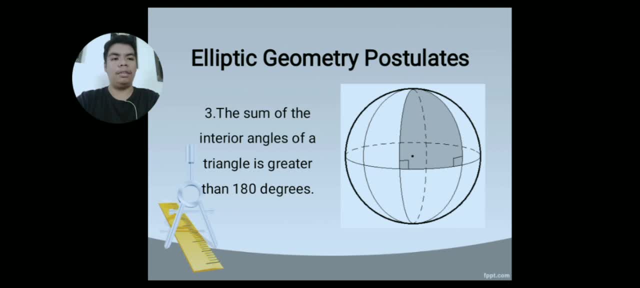 Since the ellipse is composed of curved lines. therefore, the side of the triangle in an ellipse is slightly curved. Since it is slightly curved, it will affect the measurement of the triangle And if we are going to look closely here, in the figure there are already two right angles. 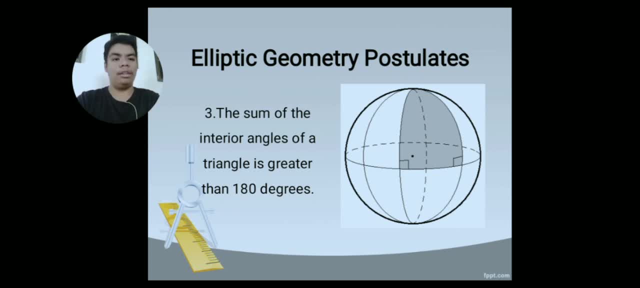 So therefore, if we are going to add that, it will already result to 180 degrees Plus the top angle. So therefore, it is always greater than 180 degrees, Assumingly that the top angle is even 101 degrees.